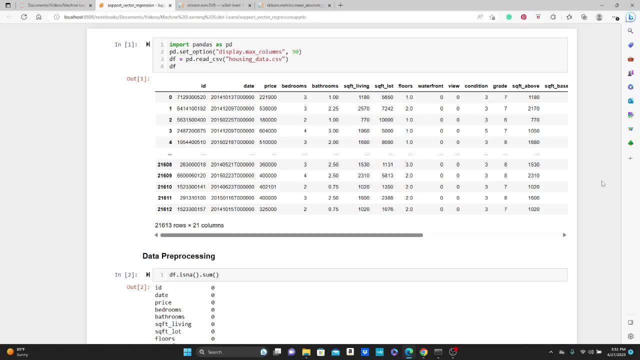 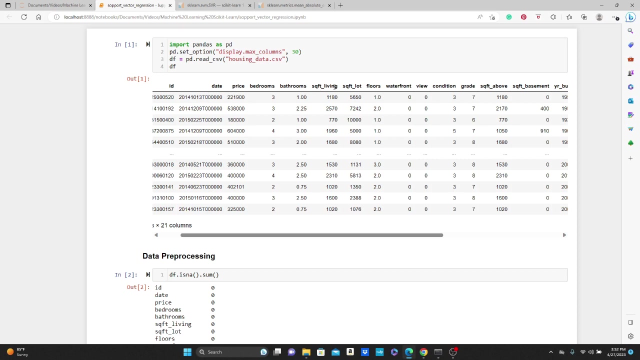 hello everyone. this is rashida. welcome to my channel. my today's video is going to be another support vector machine tutorial. this time it's going to be a regression problem. this is the housing data set we have and we are going to predict the house price based on rest of the data here. okay, we have all the data, like bedrooms, bathrooms, square foot. 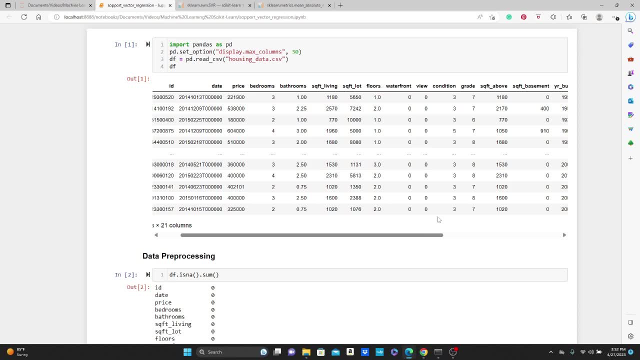 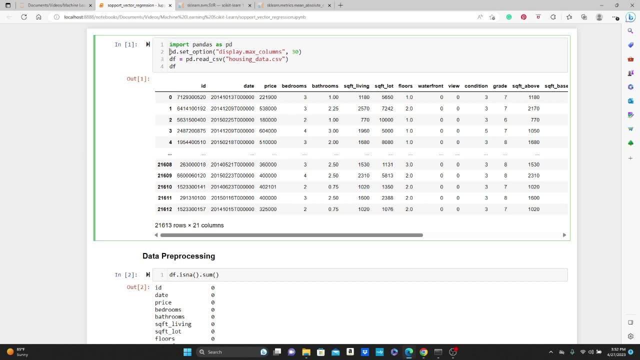 living square foot, parking lot floors, waterfront and lots of other stuff here. as usual, i'm going to start with importing pandas and then i import the data set using the pandas library and convert it to a data frame. pandas data frame. okay, and here, period set option. i set displaymax, column 30. 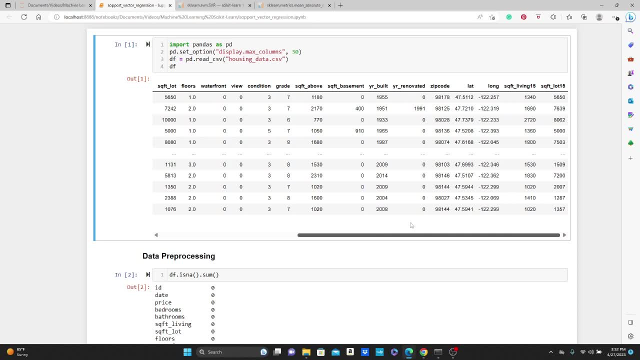 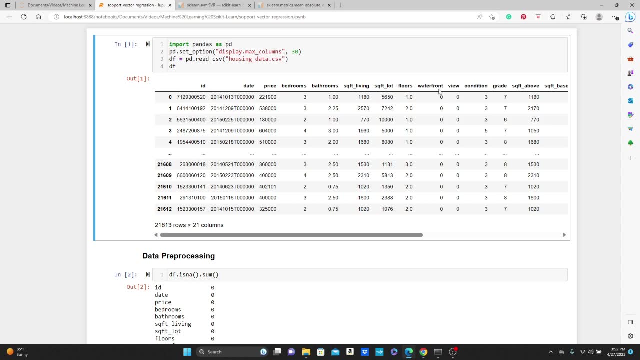 so that i can see all the columns and column names and their data type, everything. sometimes we don't see all the columns. you see the dot dot up here. that dot dot comes in between the columns and then we don't see all the column names, but it 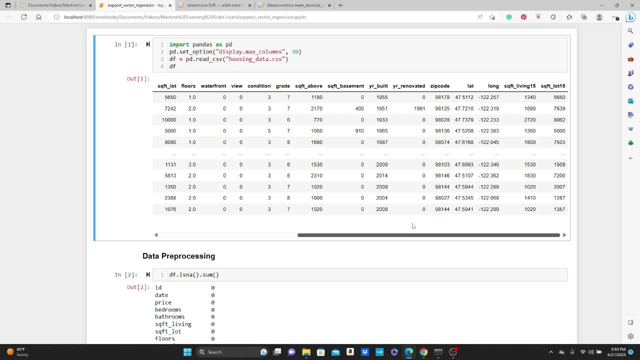 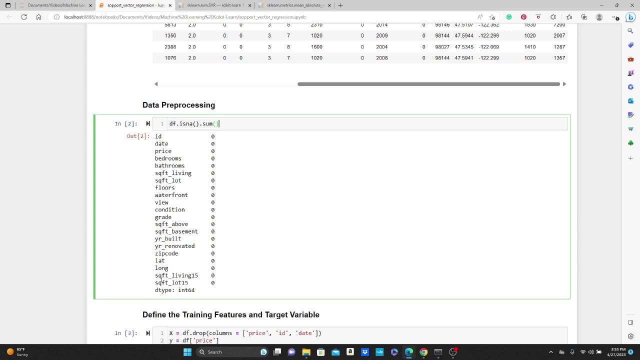 is important that you check all the data, at least see once how the data looks, if too many null values, if some data types are not right, it is good to eyeball your data at least once, and next we can check if we have any null values in our data so you can see that there is no null values. 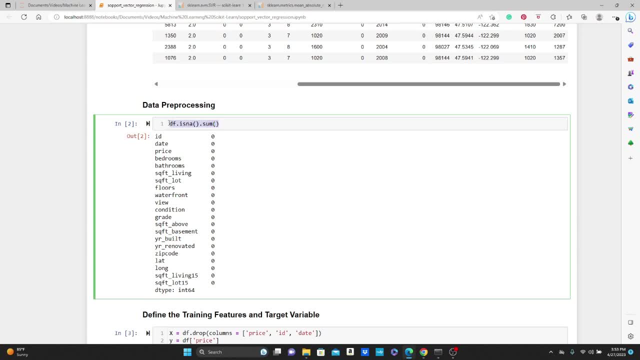 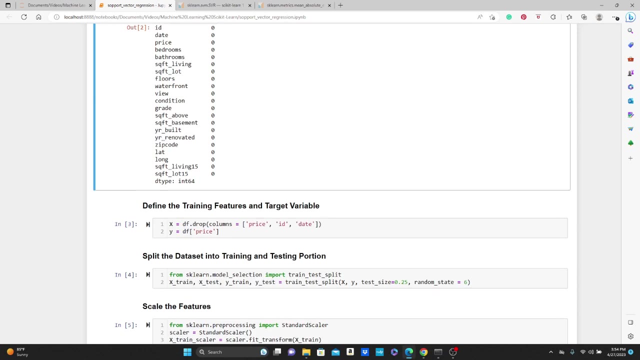 df dot is an a dot sum. that gives you how many null values we have in each column or each feature of the data frame. okay, you can see all zeros. so there is no null values. we are going to define the features and the target variable. as i mentioned already, the target variable is actually the price. 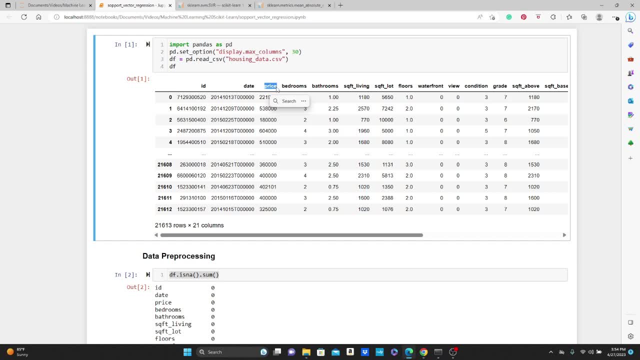 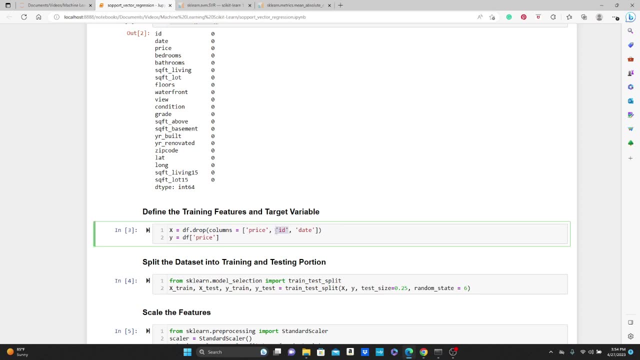 data is here. so this is our y, the target variable, and the feature- the training features- is going to be definitely not the price, because that's the target variable and we do not need the id and the date, simply because id is not related to the price. as you can see, id is just a random number in you. 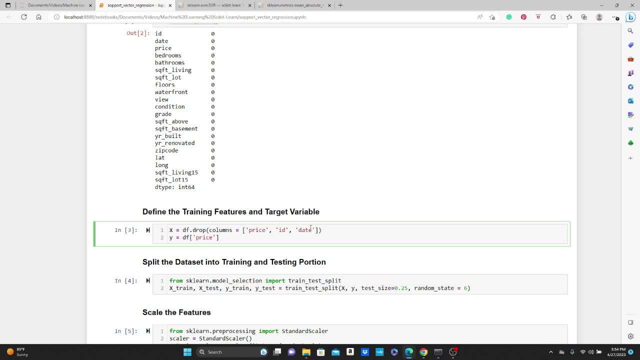 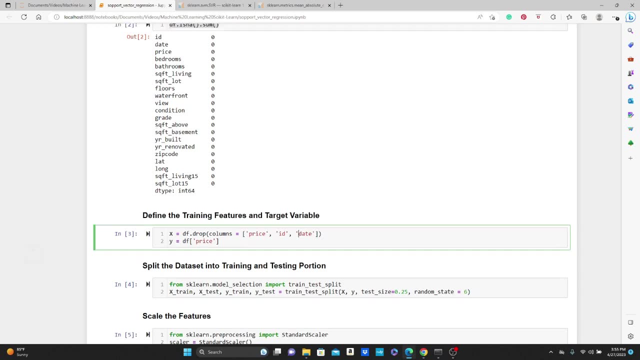 if you do a regression problem where you are doing a time series, analysis date is very important, but for this one we are not going to include the time series. instead, we will focus on the features of the house to determine the price. okay, so i'm going to omit. 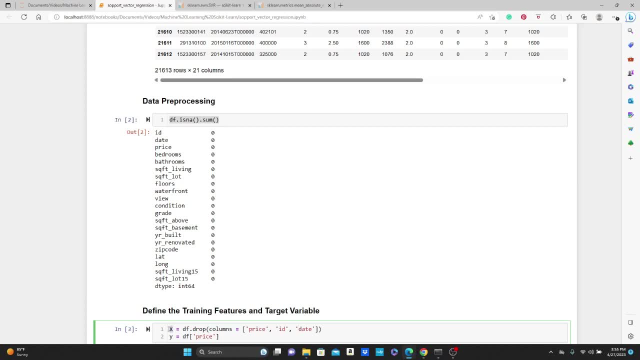 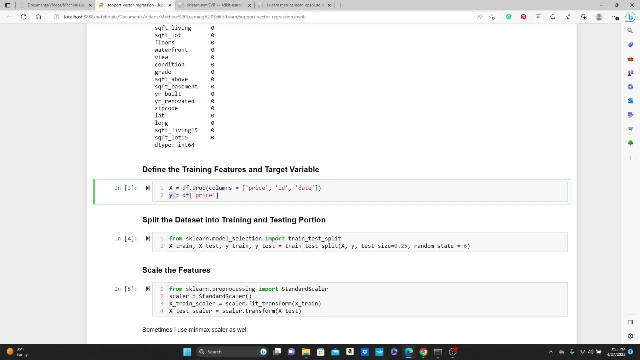 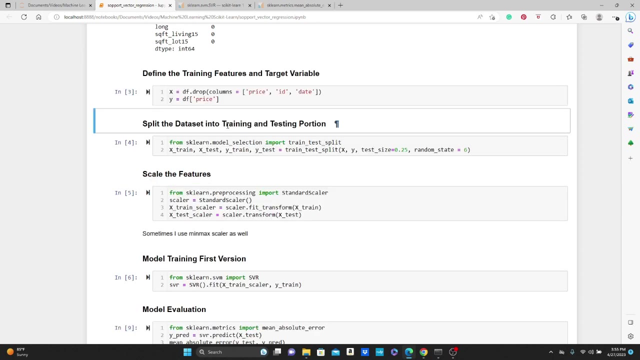 price, id and date. so that is going to be the training features and, as we mentioned before, the price is our target variable. target variable means we are going to predict price. this is a very common practice to split the data set into training and testing portion so that we can. 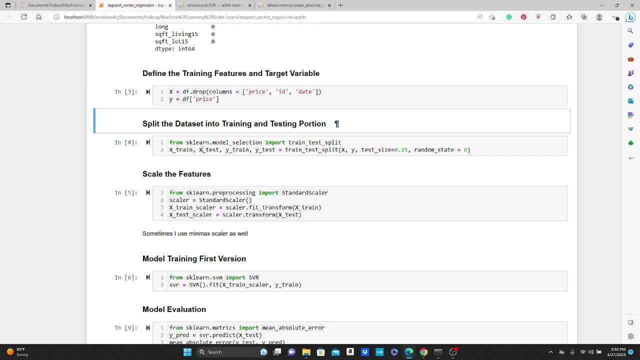 train the data set on the training portion, and then we have some data separated so that we can test the model on that data. okay, so here, uh, scikit-learn library has trained test split method for that, and first we import the train test split method and then we do x train, x test. 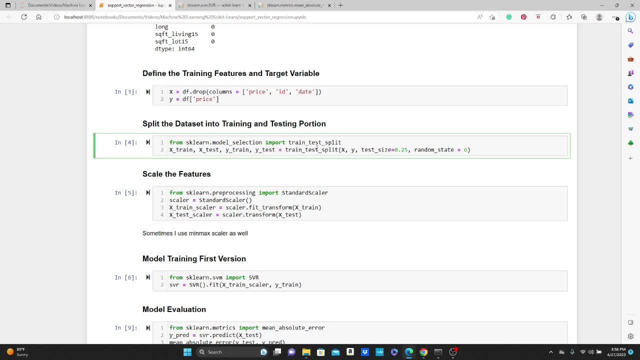 y, train y test. we call the train test split method and the parameters will be x, y and the test size 0.25. that means we are keeping 25 of the data for testing purpose and this random state. this random state can be 6, 9, 0 or 45 or 89- any random number. so let's put random state. 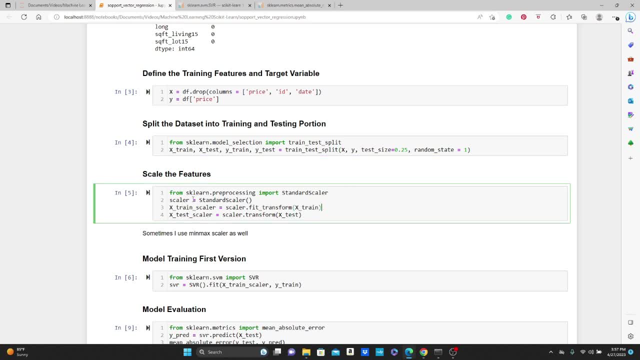 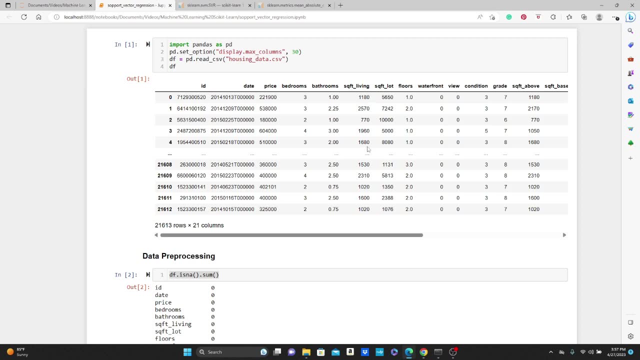 one. the next state: we have to scale the features. why do we need to scale the features? let's see, look some of our features. the numbers are pretty big. you can see five thousand, seven thousand, ten thousand and some of our features. we have a really single digit number like three, four, five, right. 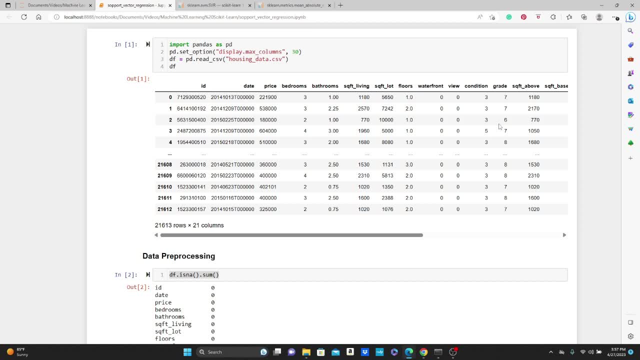 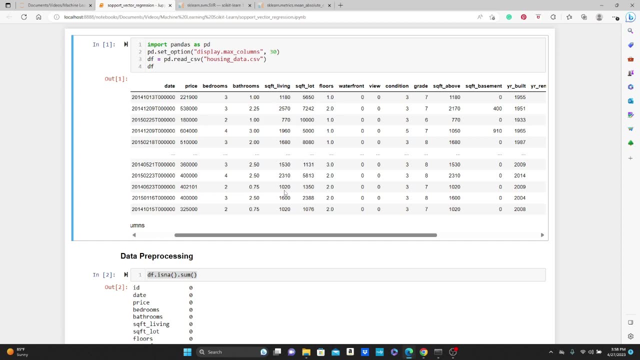 so when we have this kind of different range of data for different variables, what happens? the features with this big data can be overwhelming or they can dominate the model, and we don't want that and we want the model to recognize all the features equally. so to achieve that, we should scale the 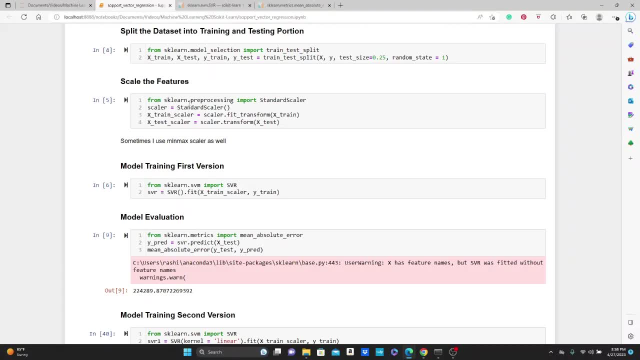 data so that all the data scales in the similar range. so for that from scikit-learn library we are going to use a standard scalar. first we import the standard scale, then we call the standard scalar function and for training data we fit, transform the training data, and for testing data we only transform. 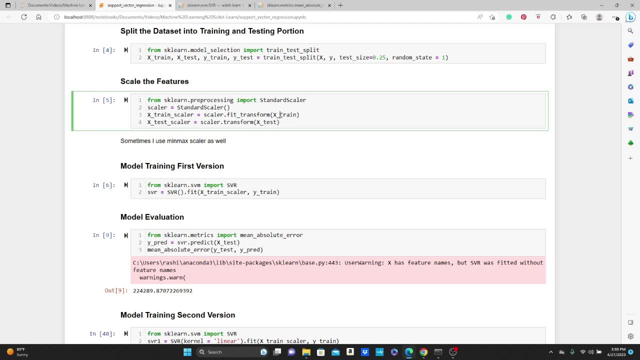 so why we do that and transform training data? because when we fit the training data it calculates the mean and standard division of the training data and for the testing data it uses the same standard division mean from the training data. because you don't want our model to know anything about our. 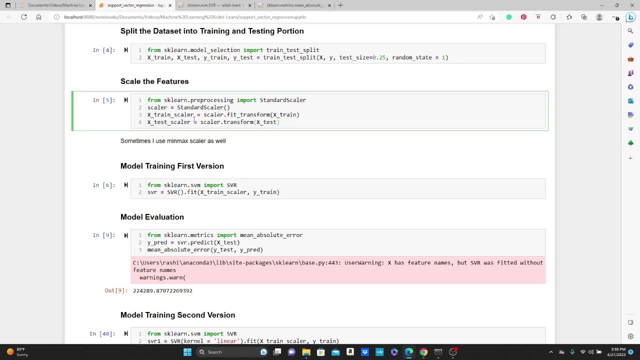 testing data beforehand. okay, the testing data is strictly kept for the evaluation purpose. so we are not giving our model any data or any information about the testing data. so that's why we do not fit our testing data. we only transform it using the information we get from the training data. but data? 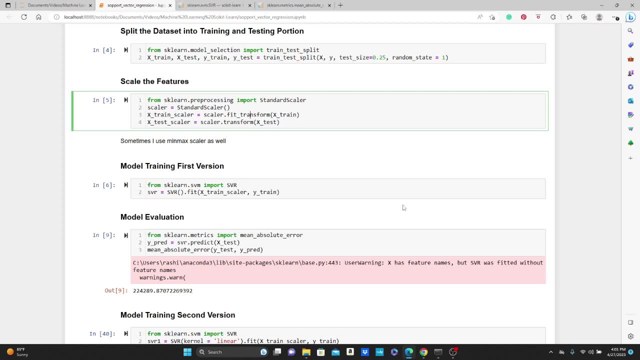 preparation part is done, let's start the training part. so for the training part i'm going to first import the support vector regressor from the support vector machine, then i just call sbr and then fit x, train the scalar after i scaled it while trained. that's all we need for training and you can see i'm 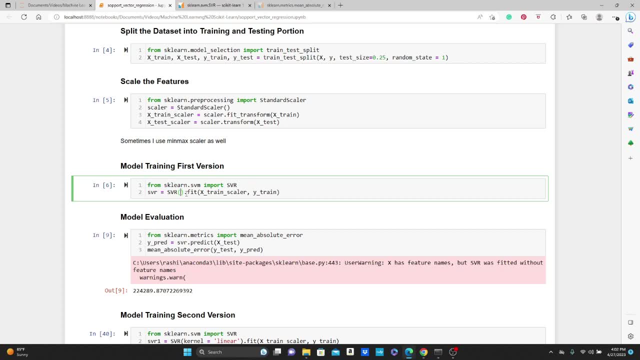 keeping it's totally empty. that means i'm accepting all the default parameters. we are not going to give any parameters to sbr, so let's see what happens with all the default parameters. as you already know that for the regression problem, we just cannot call the score function as we do for classification. 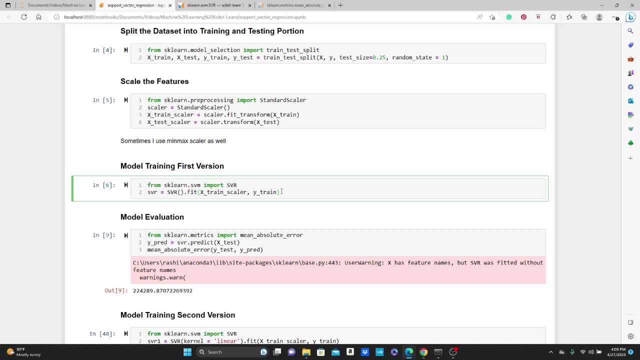 because for regression score actually does not work as evaluation purpose because it's very unlikely that you can predict exactly the same uh as as our original data. so if you call the score it's definitely going to be very poor. so that's not a good evaluation metric for regression. for regression usually we do mean 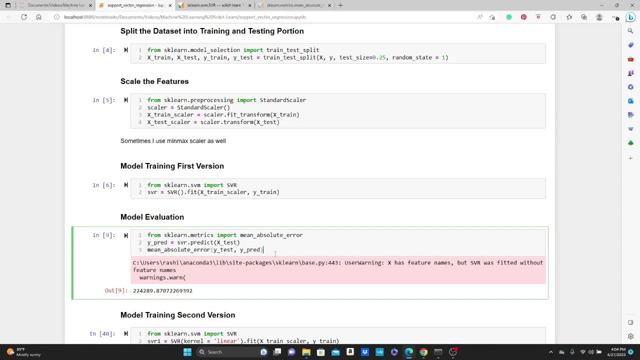 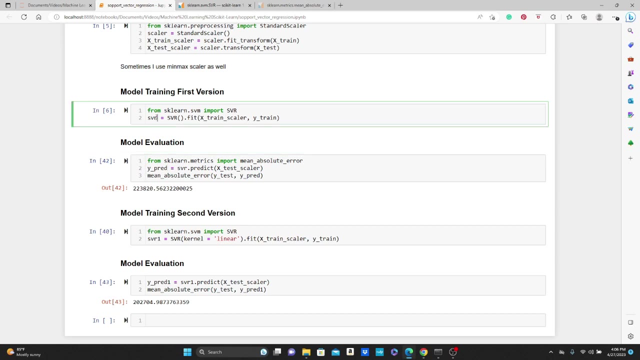 a square error or mean absolute error. that's very common. that's very common. you can also do r square, but today we are just going to check the mean absolute error here first. i predict the label using the sbrpredict. the svr is the model we already trained, so this is the svr i'm using here. 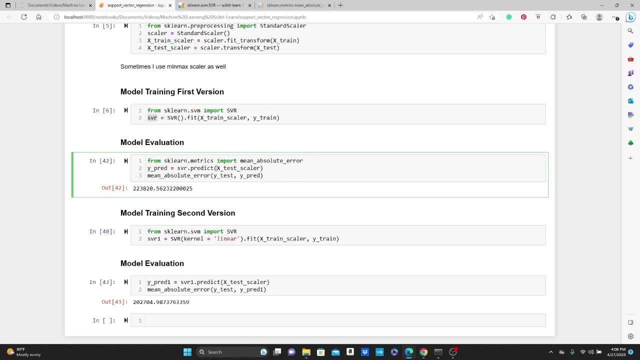 to predict. uh, the label for x test that we kept separated before for evaluation purpose and, if you remember, we already scaled it using our scalar, so x test scanner we passed here and then mean absolute error. we pass a void test. that is our original label for the testing data. 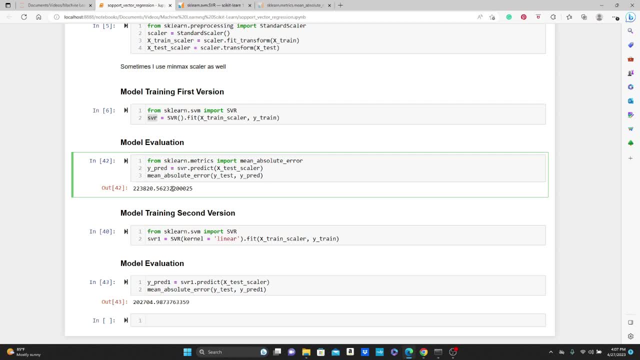 and the prediction vibration, and you can see this is our mean absolute error. now let's check and train the model again just to see if we can somehow change this mean absolute error or we can improve the model a little bit. so this time i used a kernel- kernel. 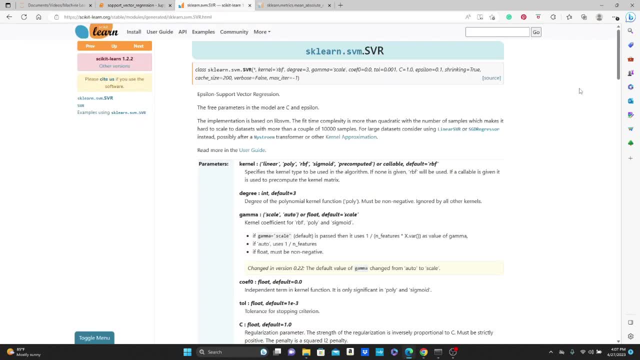 default is rbf. you can see here in the documentation we have these different kernels. you can use linear polyrbf and you can see the default is rbf and i'm going to use linear here. and there are other stuff as well. you can see, not all the parameters are for all kinds of all. 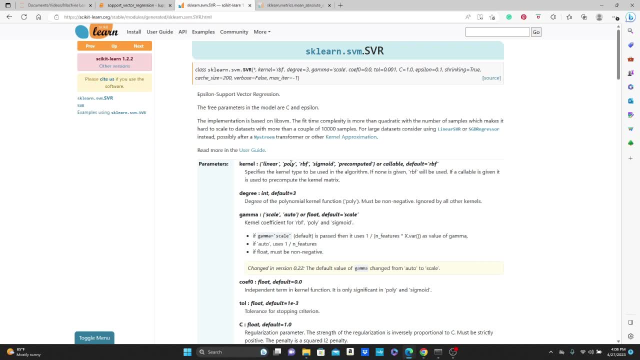 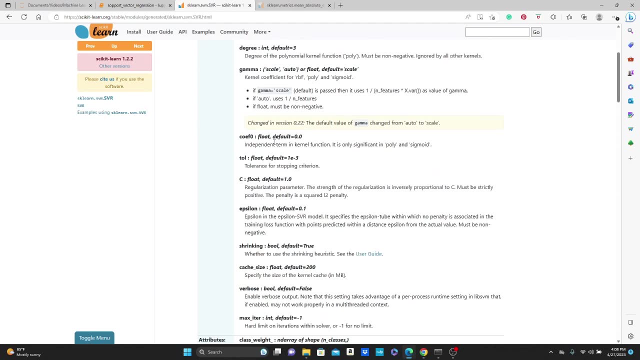 kinds of kernel. you can see dv3. that's only for poly. okay, if you do the polynomial kernel function and then you can see the efficient is for poly and sigmoid only and then you can see c is very important. parameter default is one. we are just keeping it as one and i'm just ignoring the other one. that means i'm just 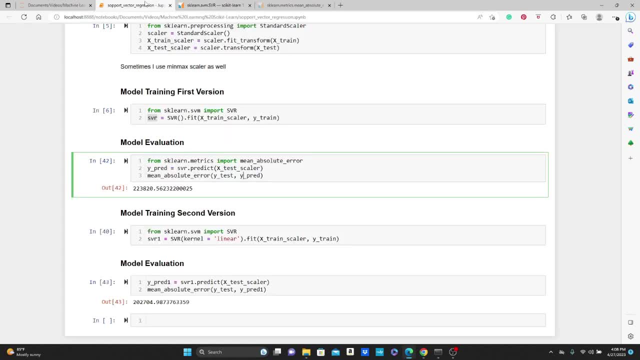 accepting the default for the other ones. okay, so i'm just changing the kernel as linear, so x train, scalar and y train again, and then i am calculating the prediction using svr1 that we claim using kernel linear. okay, so i'm using that svr1 to predict the label again.